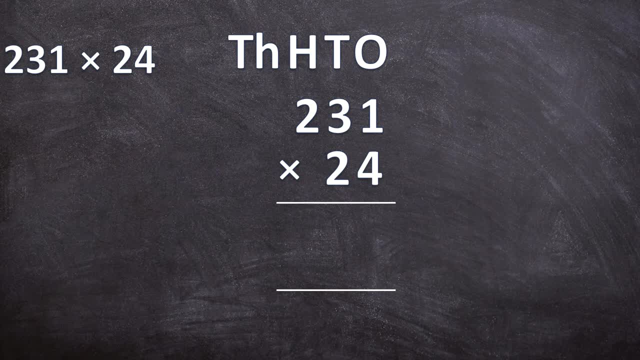 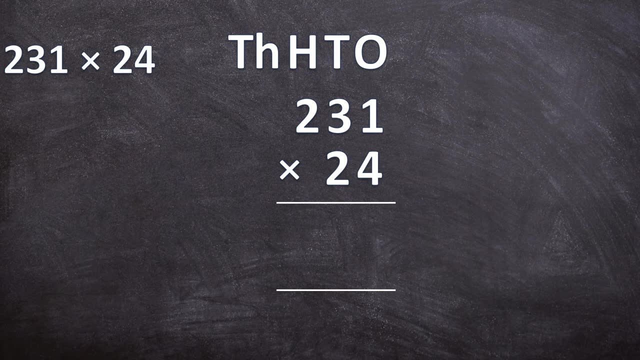 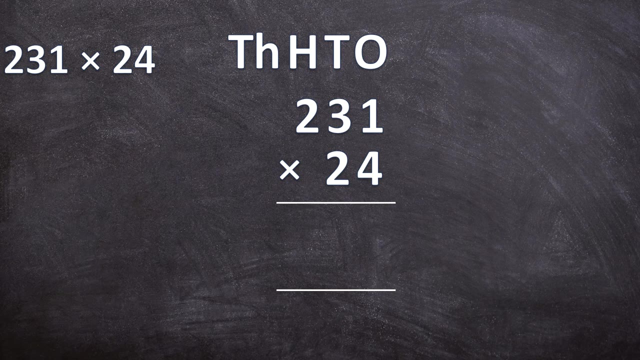 apart. you will now see why. so when we start, we take the bottom number, in this case 24, and we split that number. we are separately going to multiply with 4 and 20.. first you're going to multiply the 4 with the 231 and you'll write that answer directly underneath the line. next you will 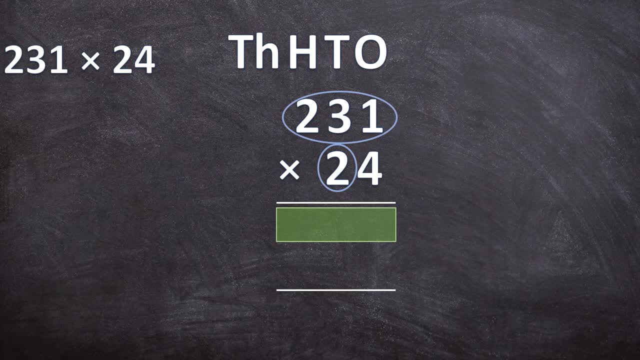 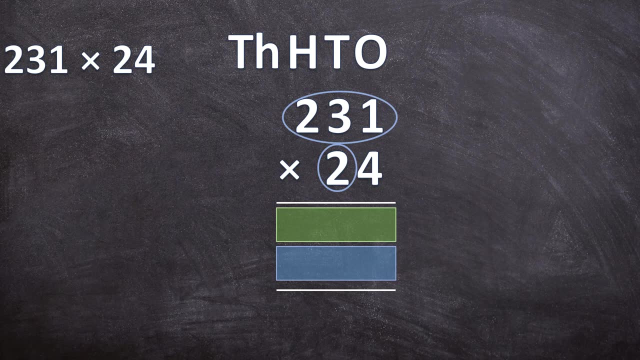 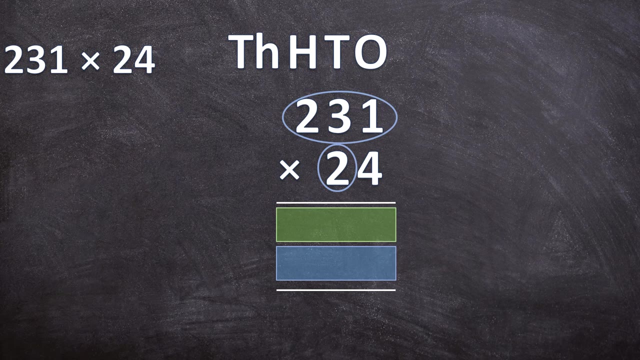 multiply the 20 with a 231 and you'll write that answer directly below the first answer you got. so now you've multiplied 4 by 231 and you've multiplied 20 by 231. all you have to do now is add those two lines together and then you can now write the answer directly below the line. 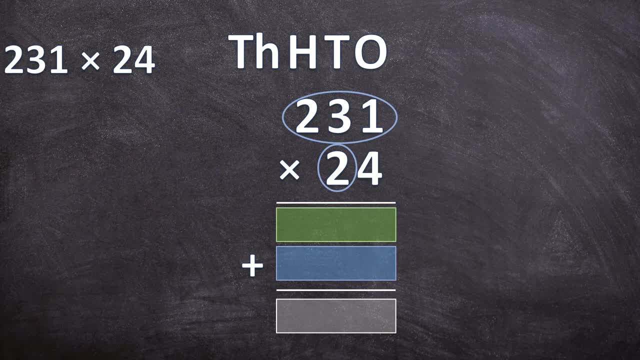 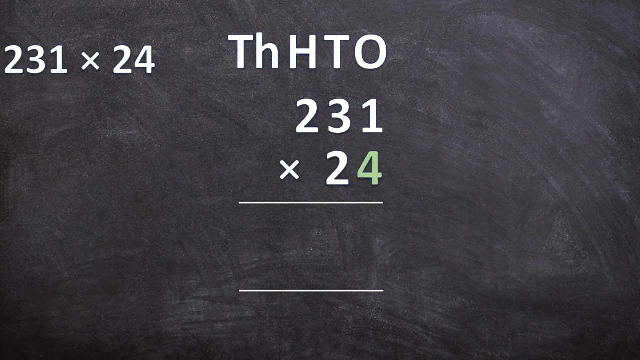 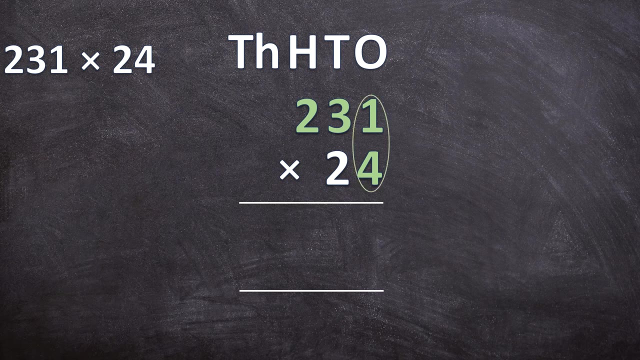 two answers together to get your final answer. So let's do this example together. First we're going to multiply with the four, So four times 231.. So we start with the ones. One times four is four. and next you're going to multiply the four with the three, So three times four is 12.. 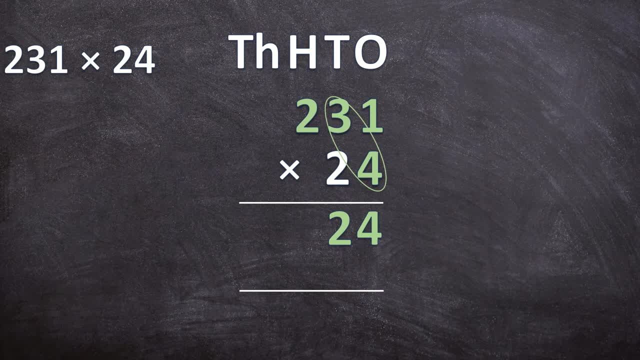 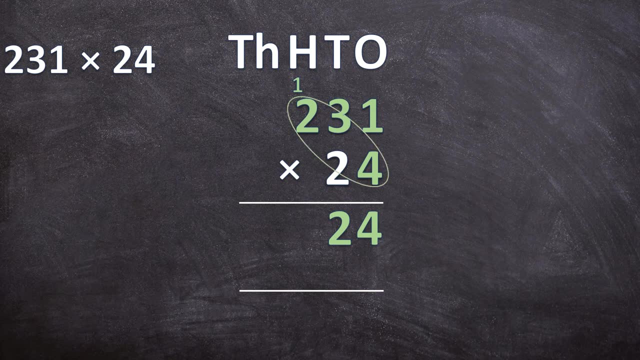 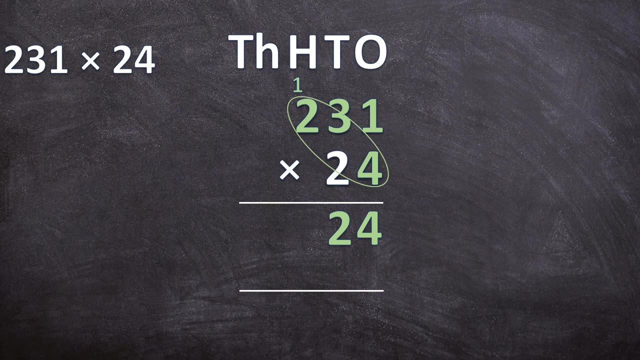 So you write down your two, but you need to carry over the one. And lastly, you're going to multiply the four with the two. So two times four is eight, but remember you carried over that one. So eight plus one is nine. So four times 231 is 924.. And now we're. 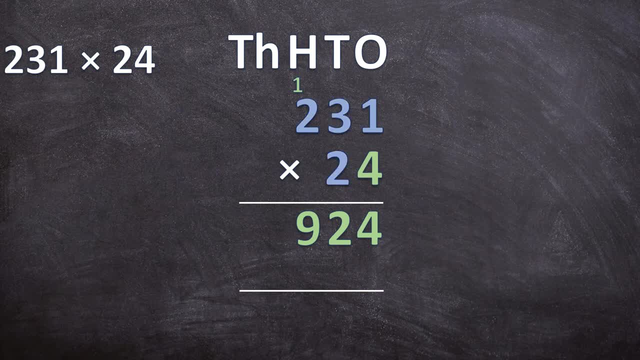 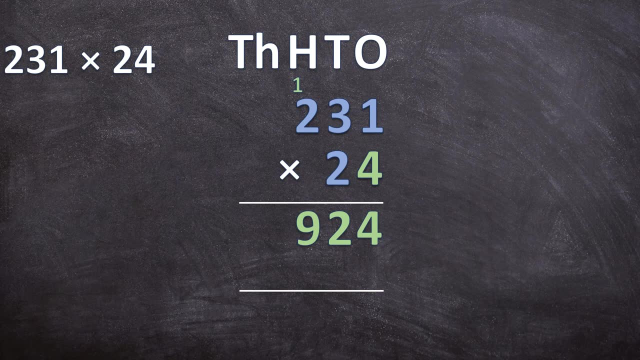 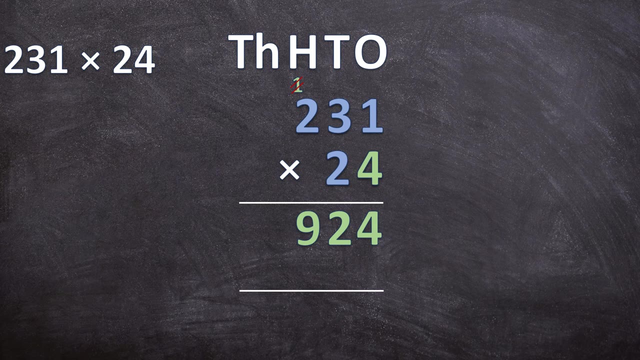 going to multiply the twenty With the 231.. But before we do that, there's two things I want you to remember. First of all, we already multiplied with the four. We need to cancel that one that we wrote above the two, because we are finished with that one. And then the next thing I want you to remember: 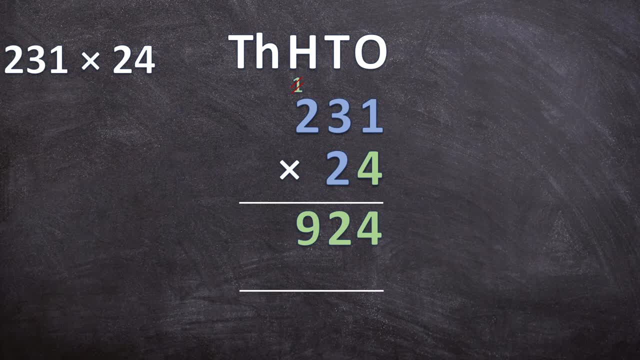 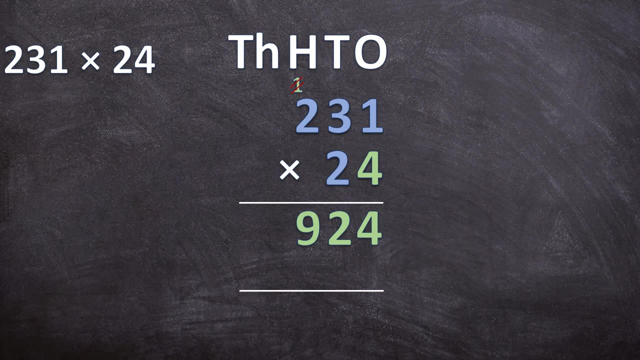 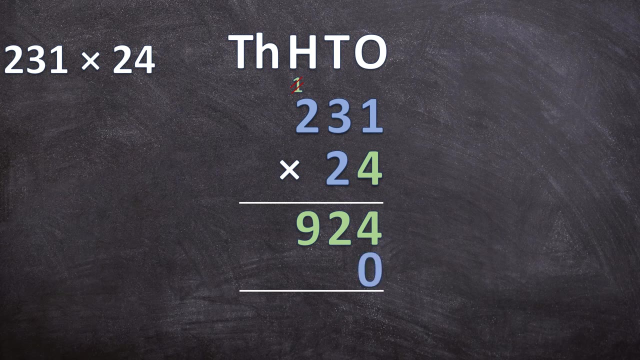 is that we are multiplying with 20 and not with two. So 20 is in the tenth place value, So it's 20 and not 2.. That is why, before we start multiplying the digits, we are first going to write a zero in the answer line. So that's to make sure that our answer is going to be 20 times 231. 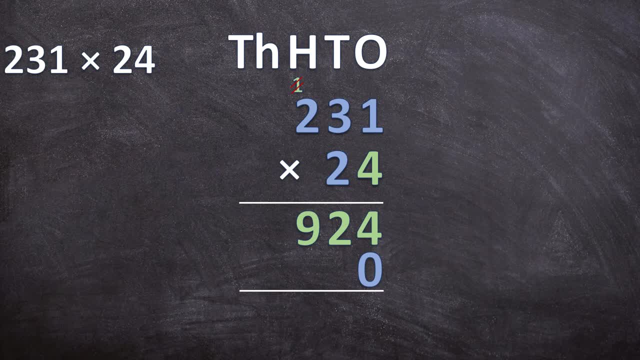 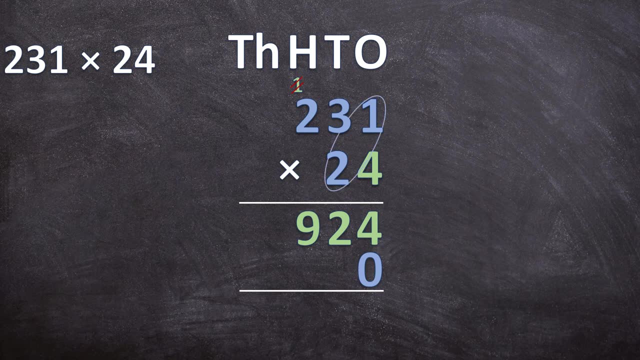 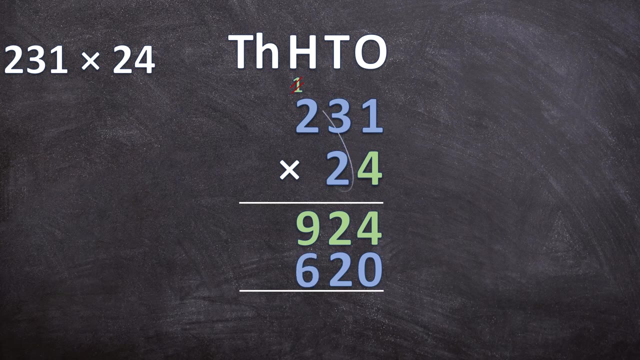 and not 2 times 231.. So now that we've written down the zero, we can simply multiply the digits. So 2 times 1 is 2.. 3 times 2 is 6. And 2 times 2 is 4.. So now you see why it's so important that you wrote down that. 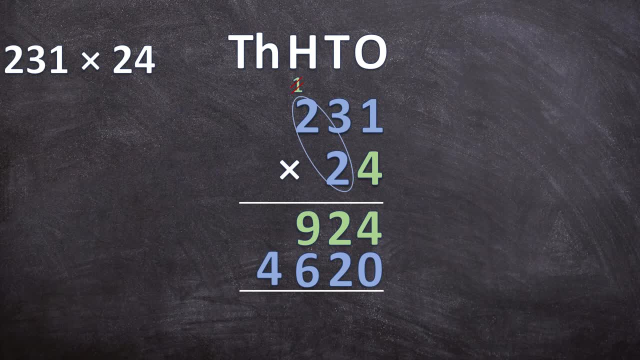 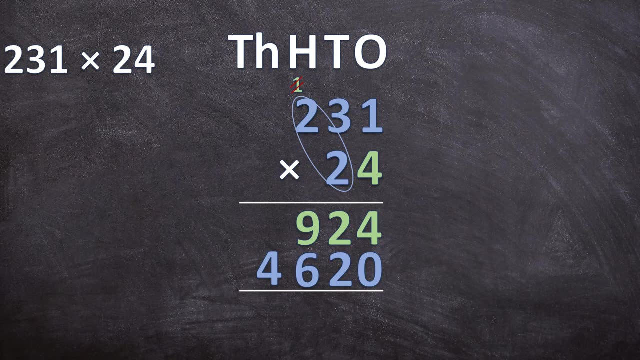 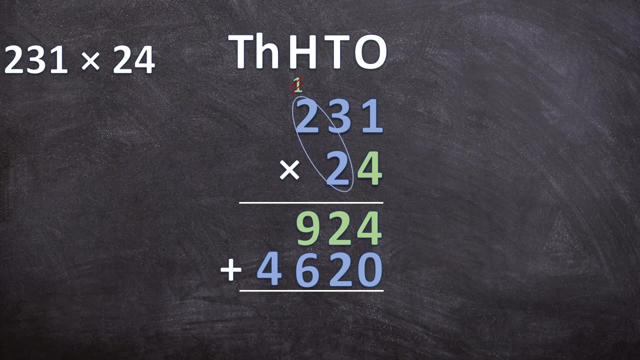 zero before you started multiplying the digits, because 20 times 231 is 4620.. We just need to add those two answers together, So let's start at the ones, like we would do a normal addition sum. So 4 plus 0 equals 4.. 2 plus 2 equals 4.. 9 plus 6 is 15.. Very obvious that. 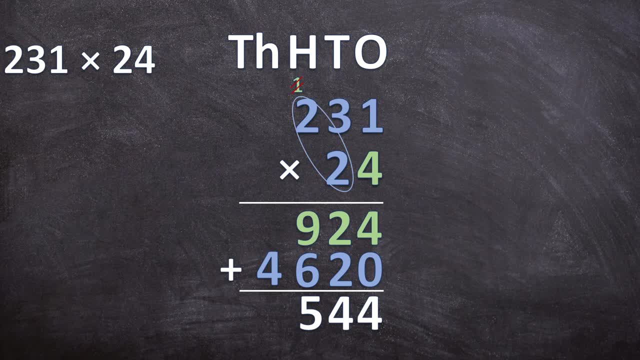 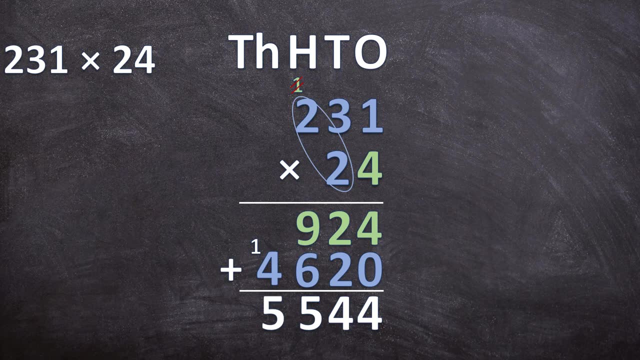 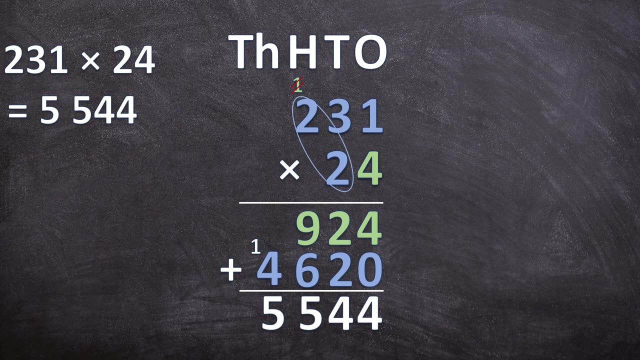 you'll be writing down your answer first, But now you will take the one over And 4 plus that. one number times a two-digit number. if you feel like you need to go and practice a three-digit number times a two-digit number some more, i will have a worksheet with a memo in the description box below. 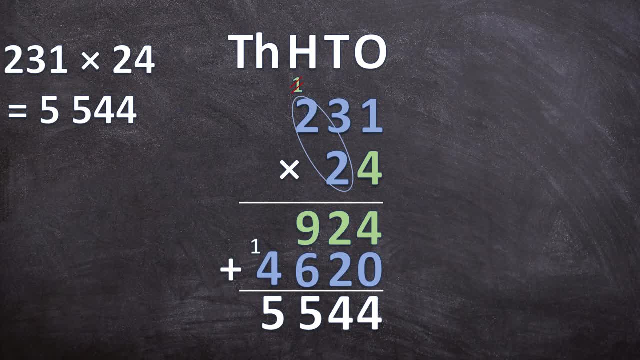 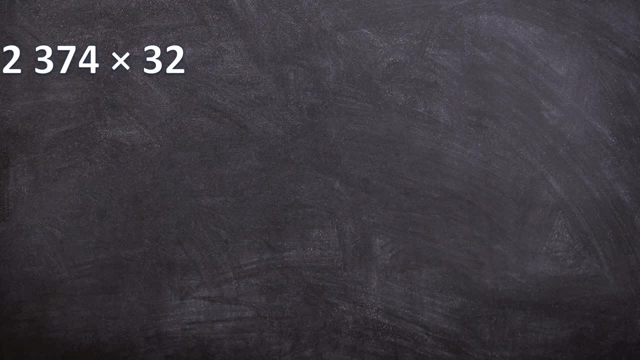 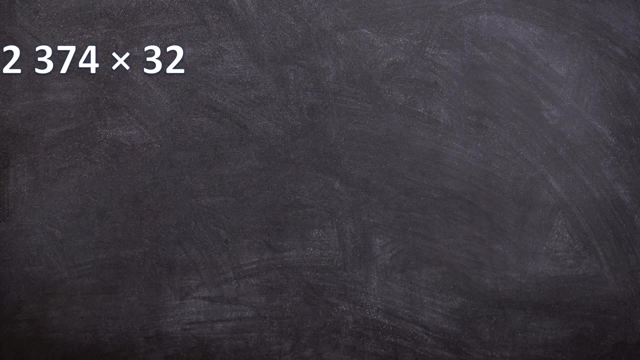 you can just click on the link and go and download it and go and practice this some more. but now let's move on. so here we have a four-digit number times a two-digit number, so 2374 times 32. so the first thing we do is we write them neatly underneath each other so that your ones are. 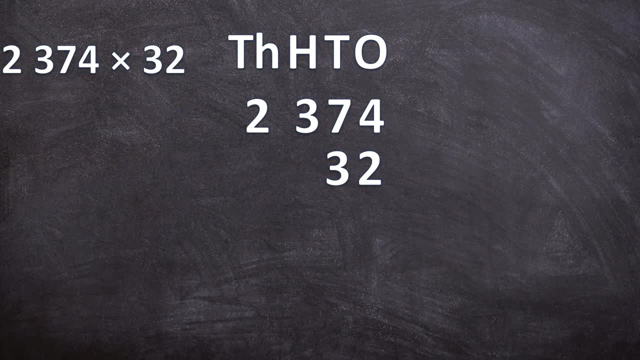 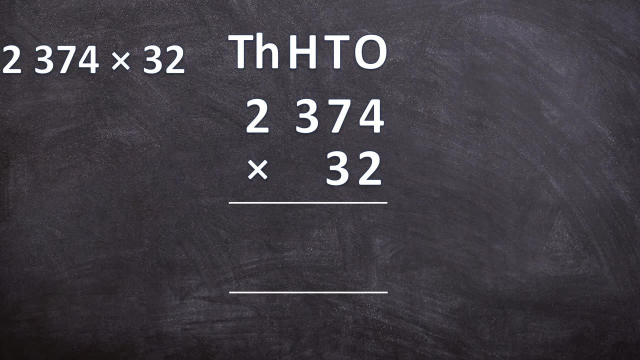 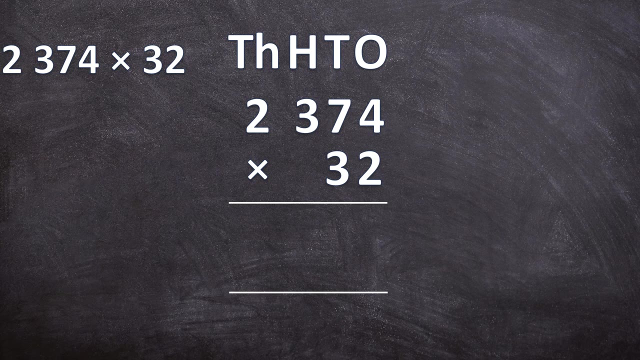 directly underneath each other, and also your tens, and then your multiplication with your two lines, and just by looking at this it can seem very intimidating. but you just do it one step at the time and you will get your final answer. so the first thing you do is you split that 32. so 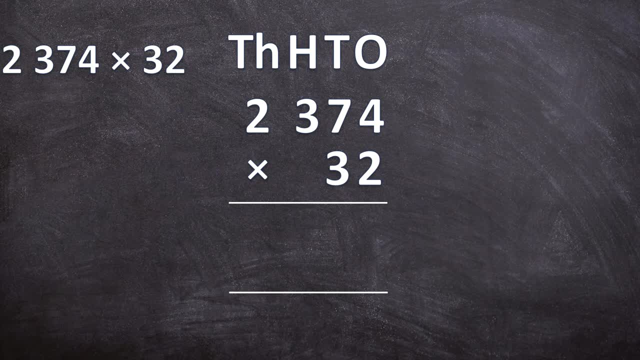 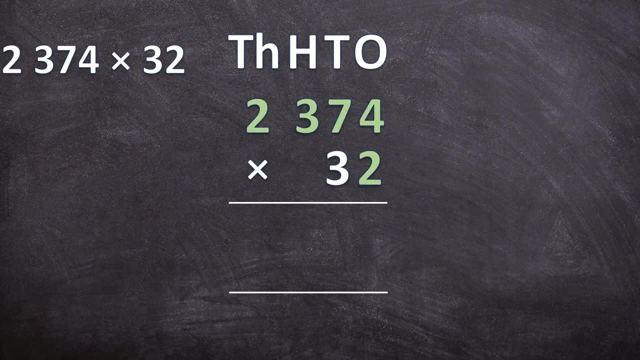 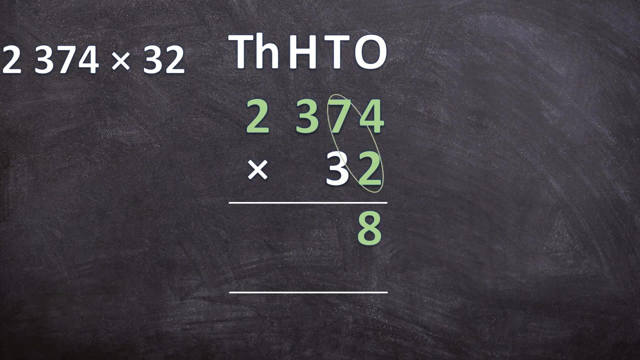 we're first multiplying with 2 and then we're multiplying with 30. So 2 times 2374.. So first we multiply the 1s, So 4 times 2 is 8.. Next, 7 times 2 is 14.. Remember, you write down the 4.. I do carry over the 1 and you write it there. 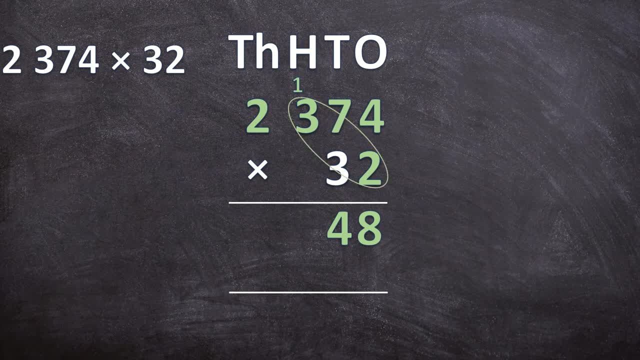 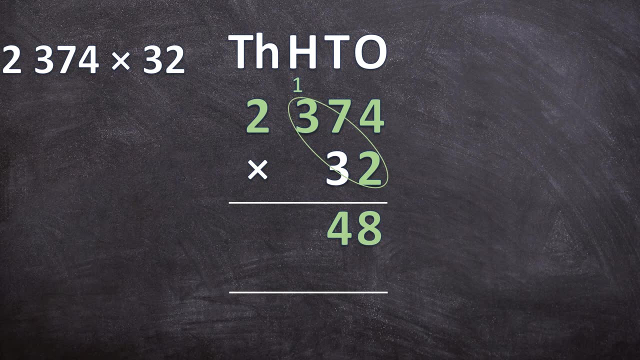 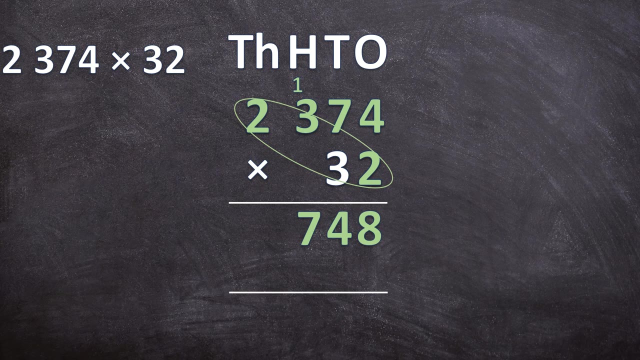 So next we have 3 times 2.. And 3 times 2 is 6.. But remember, we carried over that 1.. So we still need to add that 1.. So 6 plus 1 is 7.. And now we multiply the last two digits: 2 times 2 is 4.. 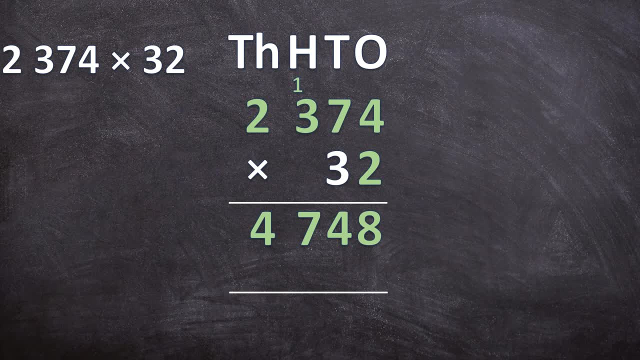 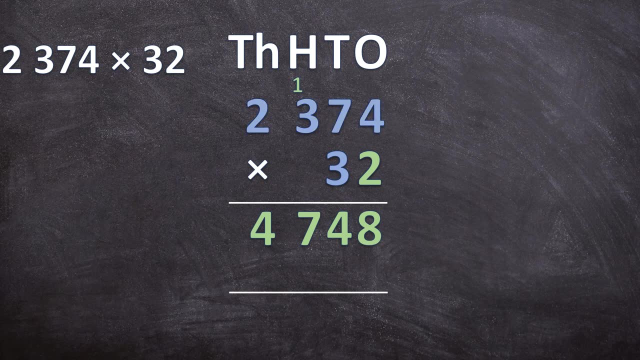 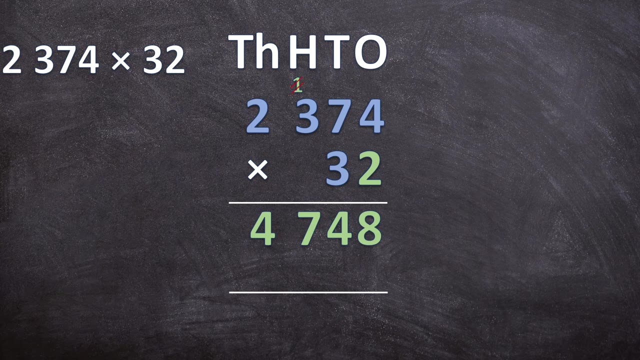 So now we move on to the 30. We already multiplied with the 2.. Now we multiply with the 30. So 30 times 2000.. And remember that we already worked with that 1.. So we need to make sure we cancel that 1.. So we 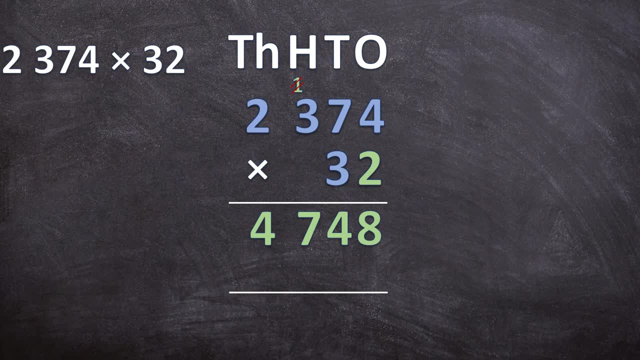 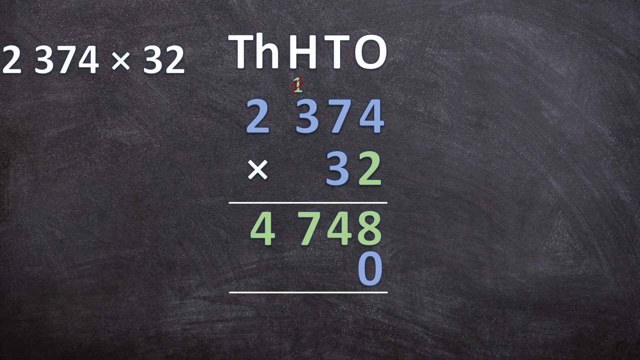 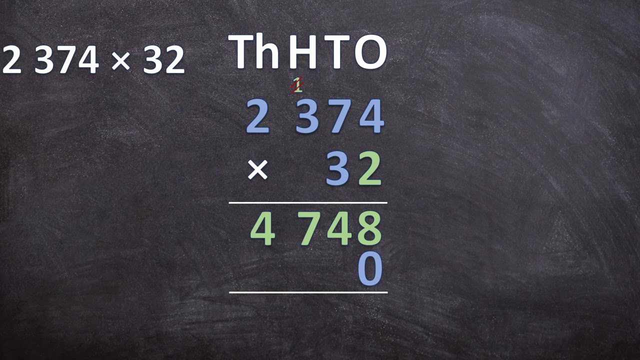 don't get confused and use it again. And now, the second thing you probably already remember is that we need to write our 0 in the answer line, Because we are multiplying by 30 and not just by 3.. So now that we're done with that, we can just start multiplying our digits. 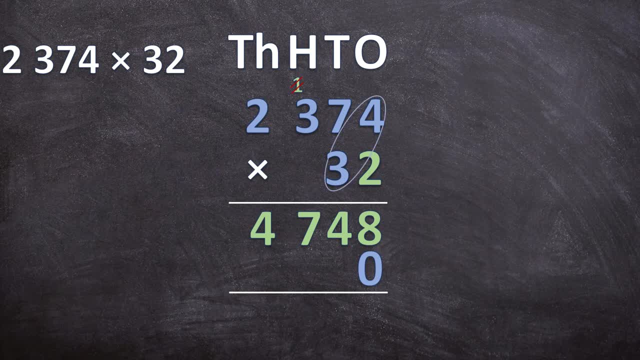 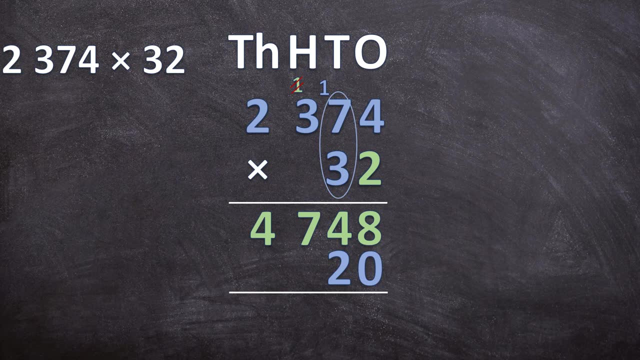 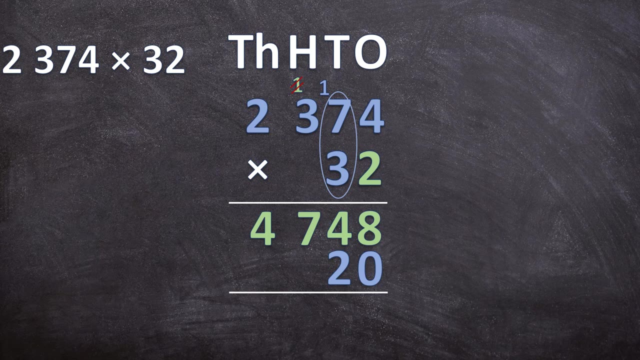 So first, 3 times 4 is 12.. So you write down your 2.. You carry over that 1.. Next is 7 times 3.. 7 times 3 is 21.. But remember, you carried over that 1. So you still need to add it. So 21 plus 1. 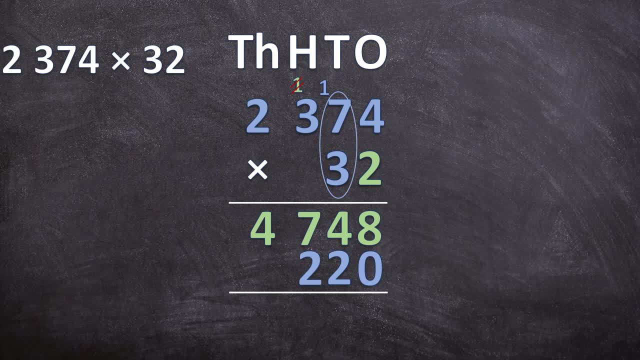 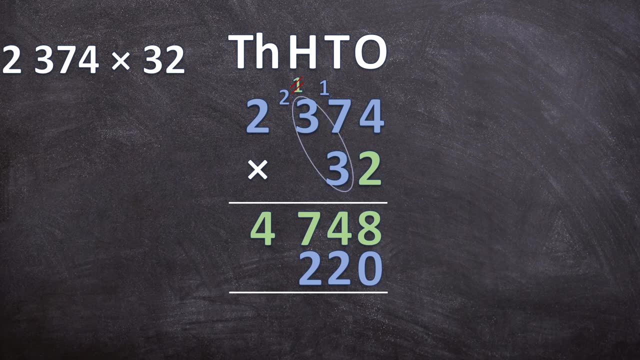 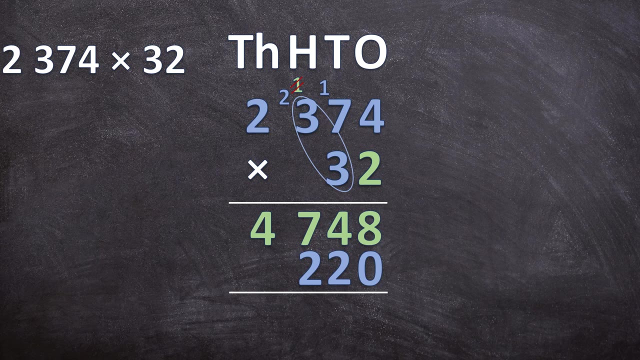 is 22.. So you write down your 2 for 22.. But you still need to carry over that 2.. Next we have 3 times 3.. 3, 3, 3 is 9.. But remember that 2.. So 11 times 9 plus 2 is 11.. So you write down the. 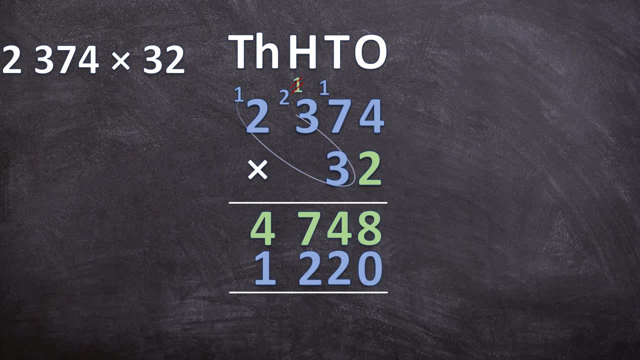 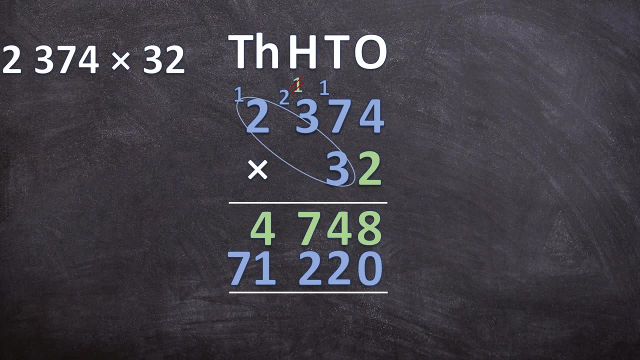 1. So you carry over the 1.. 2 times 3 is 6 plus 7 times 2 is 11 is 7.. So now you have the answer for 2 times 2. orders per digit is 2374.. 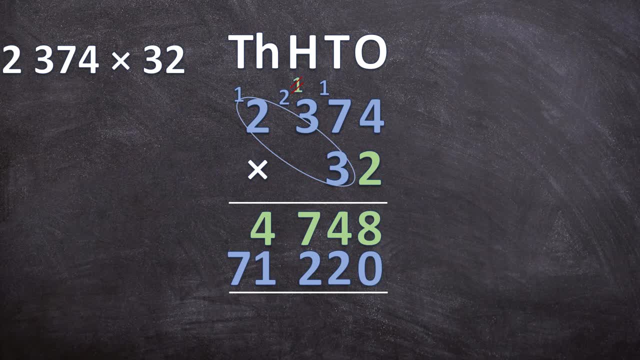 And then you have the answer for 30 times 2374.. So all you need to do next Is the U as well, So let's go with the putting off. So now we're going to multiply by 30, you carry over the 1.. So all we need to do is: U becomes 21, 3 times 2374.. So all you need to do next is: